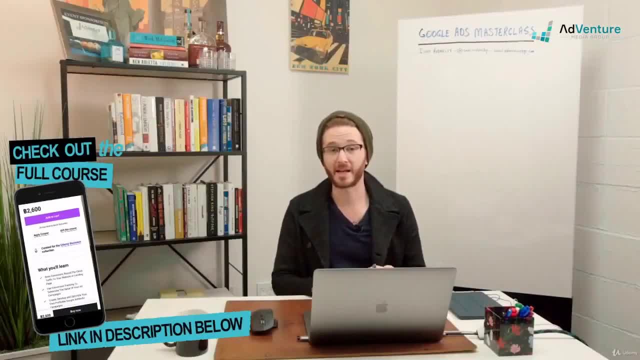 In this lecture we're going to talk about setting our daily budget. And yes, in Google Ads we set daily budgets, We don't set monthly budgets. When you set a daily budget for your campaign, you're telling Google how much you want to spend each day, the maximum you're willing to spend each day for this campaign, Google has updated a couple of things with regards to the daily budget and how it works. You can actually spend up to double your daily budget, but it won't exceed your daily budget over the course of an entire month multiplied by the average amount of days in a 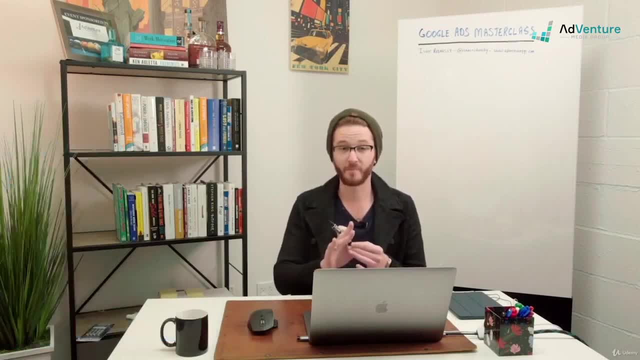 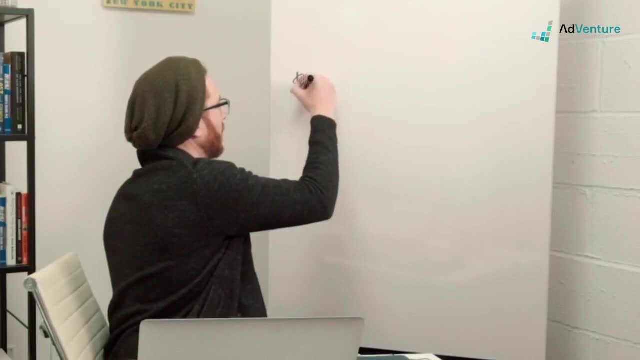 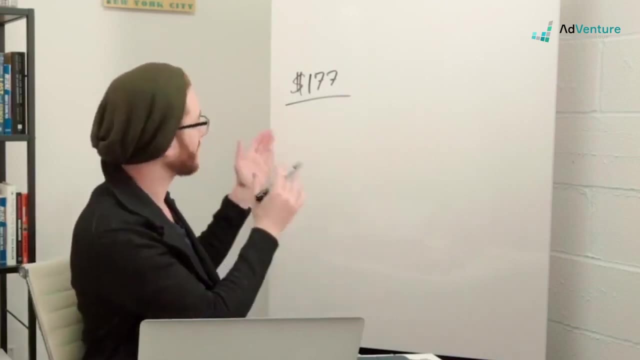 month. So that sounds a little complicated. So let's just quickly look at an example. So say, for example: say, for example, I have a daily budget of $177.. Okay, Now the average amount of days in a month. what you're telling Google is that this is what I want to spend per day. 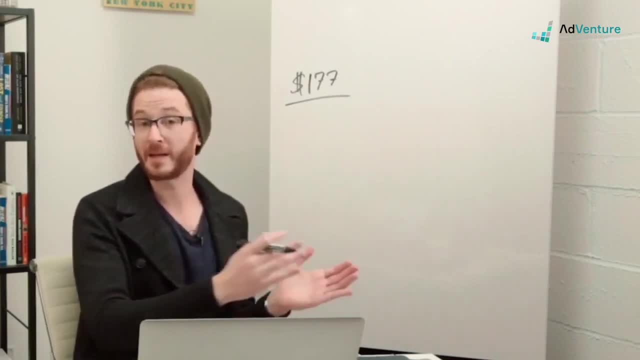 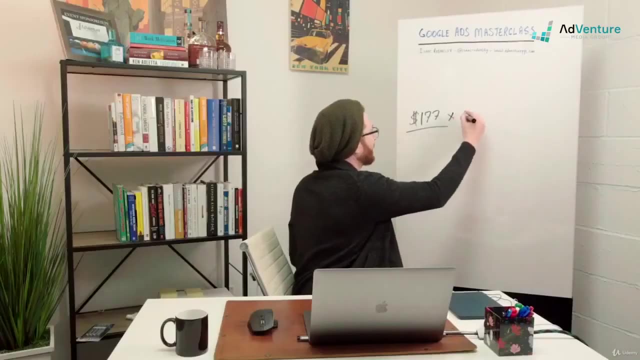 And Google will say like: okay, we get that, We might spend a little bit more, You might spend. you might spend a little bit more, You might spend a little bit less, but we will hold ourselves to that multiplied by 30.. If I take 177 and I multiply that by 30,: what do we get? Do the math: $5,310, I believe right. So $5,310 is the most you're going to spend over the course of a month, which is actually $177 a day, But I could spend on any given day. 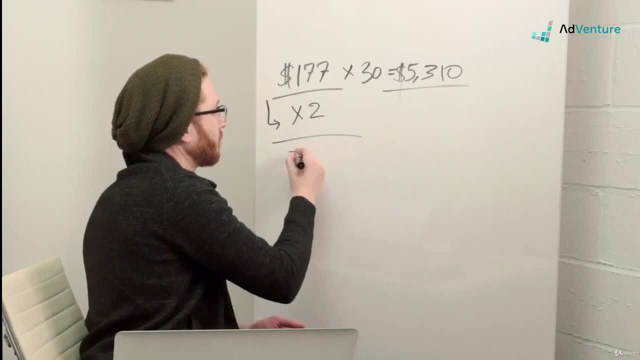 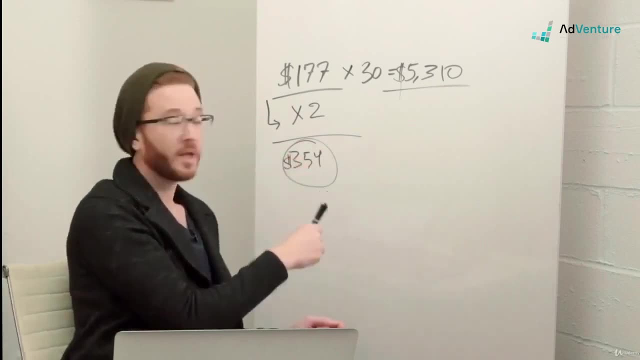 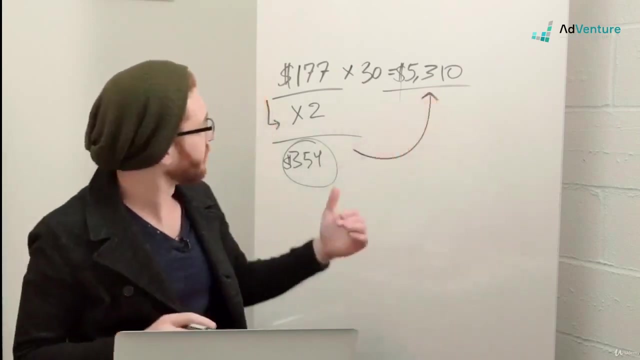 $177 up to double that right. So that comes out to $354.. Okay, So I could spend $354 on any given day, but I won't spend $354 every day because then I'm going to greatly exceed my allotted budget for the course of the month. So it's a little bit of a weird system. It used to be that Google would really not go over your daily budget. Google has changed and they will outright say that we could spend up to double your daily budget on any given day. And the reason why they do that is because they 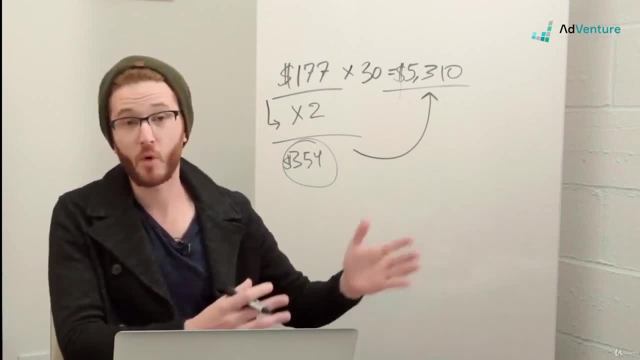 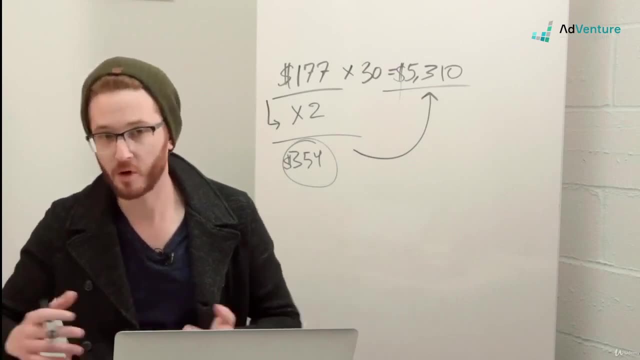 say like: okay, if on any given day we feel that you could get more impressions and more conversions and more keywords that you want to get, then we'll give those to you and we won't spend as much next week or the day before or something like that. So I actually think it's a good system And we've 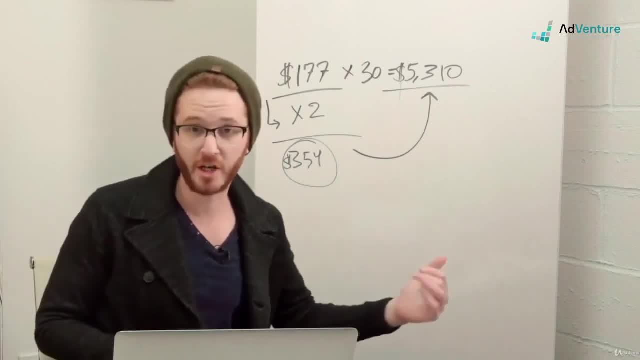 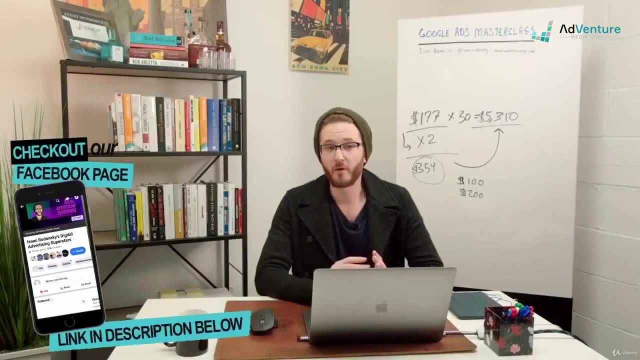 seen better results in our campaigns as a result of this change. Now, how do you determine what your daily budget should be? Okay, That's a good question. There's no way to answer that for a new campaign. The real way to go about figuring out what your daily budget should be is how much. 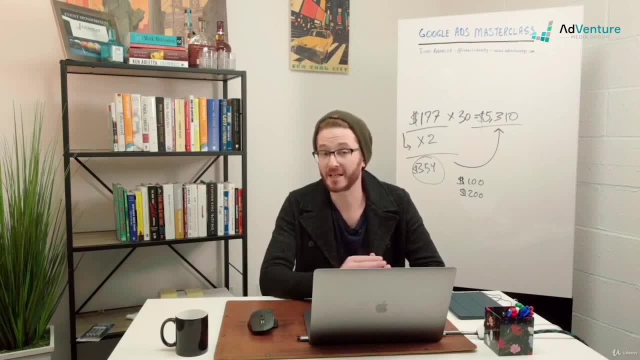 profit do I need to earn? What return on ad spend do I need to generate for these campaigns to be generated? And remember, what we're dealing with here is salesmanship in pixels. Salesmanship is all about making a profit, And we've said this before. I'll continue to say this again: Everything. 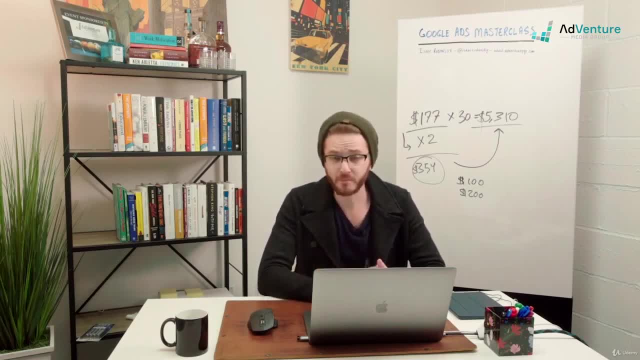 we do, every decision we make must be anchored to our desire and our ultimate goal for profit. But if you're creating a campaign for the first time, then there's no way to really know. So if you have a budget behind you and you're able to invest in testing what's going to work. then put a daily budget that's appropriate. And if you have a budget behind you and you're able to invest in testing what's going to work, then put a daily budget that's appropriate. And if you have a budget behind you and you're able to invest in testing what's going to work, then put a daily. 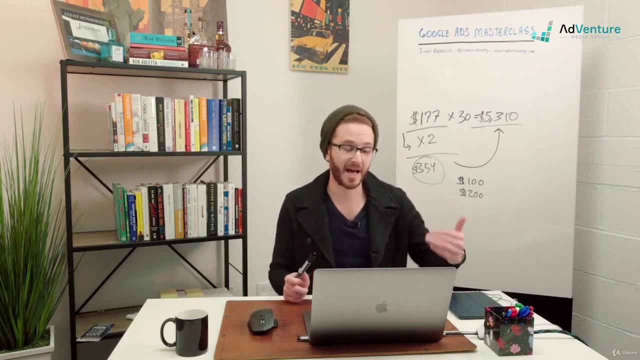 budget that's appropriate. And if you have a budget behind you and you're able to invest in testing what's going to work, then put a daily budget that's appropriate. So I can't tell you what that is, Whether it be $50,, $500, or $5,000, I don't know. It could be $10, it could be $1. I mean. 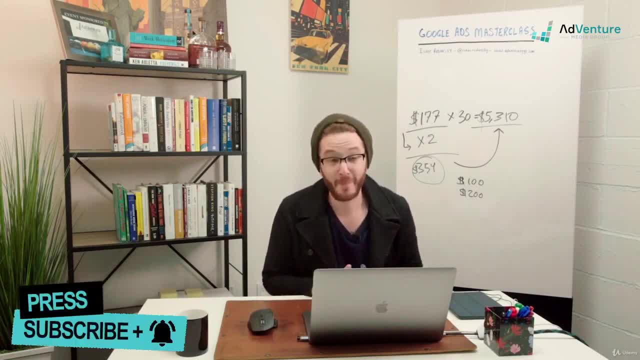 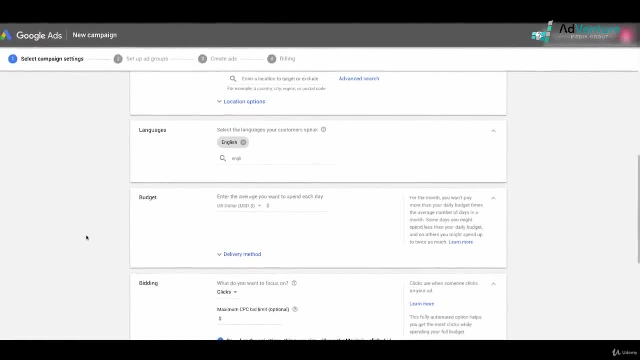 I don't think it's worth getting involved in the campaign at $1 a day. I would say at minimum $10 a day, spread across one or two keywords at most. So in our case, for now, I'm just going to put in a quick $50 a day budget. It's a test account And again, remember that this is just 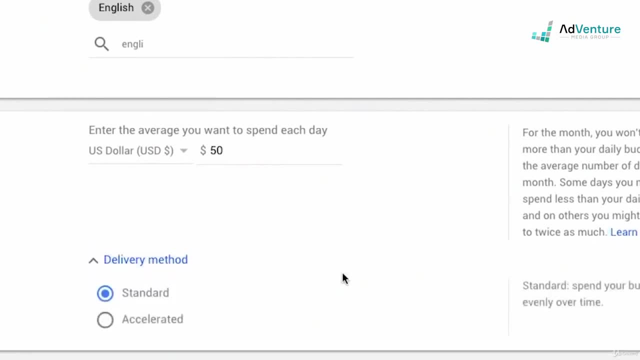 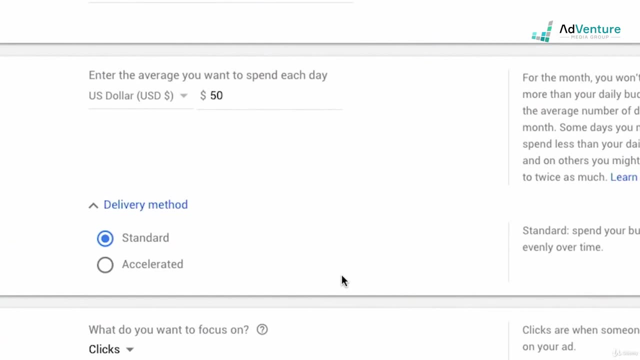 for this campaign. And now I'm going to delivery method. If I twirl down delivery method, which is an advanced setting, we have two options: standard delivery method and accelerated delivery method, And I want to jump into a slide to explain exactly how this works. 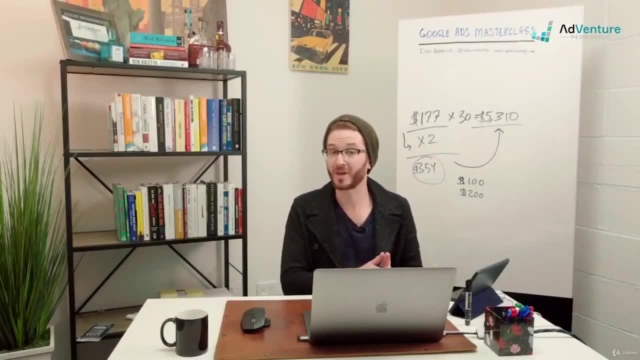 How do you want us to deliver those impressions to you? Do you want them all at once? Do you want them as fast as possible, Or do you want them throughout the day, or throughout the maximum amount of time you have given your ad scheduling options? So let's see what that looks like. So, 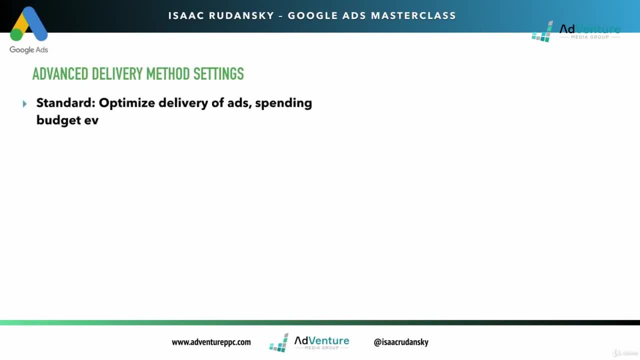 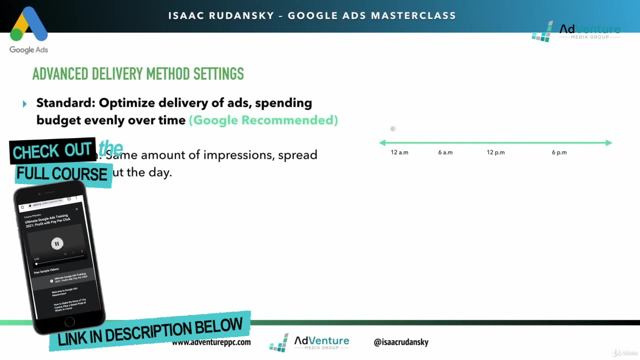 advanced delivery method. when you click standard and when you choose standard as an option, you're optimizing the delivery of your ad spending budget evenly over time. That's what Google recommends. The translation of that is the same amount of impressions spread out throughout the day. So here's a visual representation of that looks like. Let's say I'm bidding from 12 am to 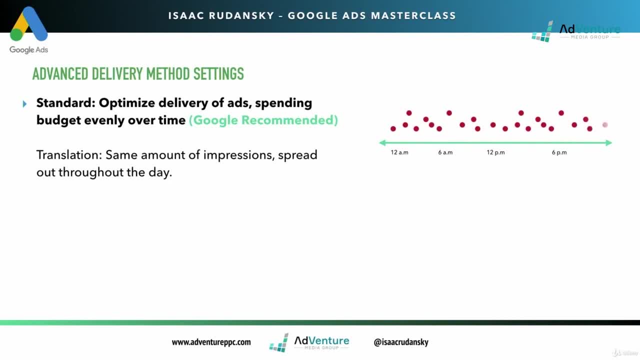 12 pm. I'm bidding 24 hours a day. My impressions will be a relatively even distribution throughout the day. So if Google knows that I'm going to get, for example, if Google knows the maximum amount of impressions that I can get is 2000 impressions, they'll stagger those impressions. 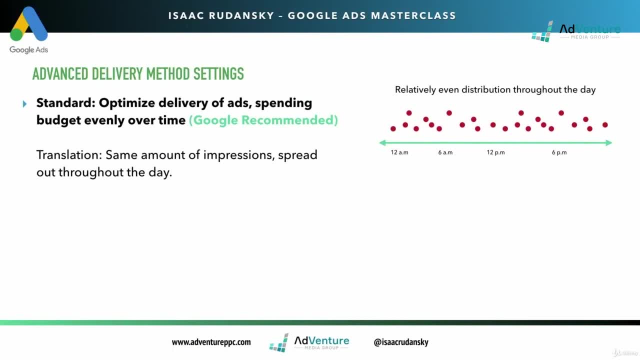 throughout the day, So I'll miss out A bunch of auctions early, and Google has enough computing power to know exactly how to give me that even distribution. If I choose accelerated delivery, I'm not optimizing the delivery of the ads. I'm spending my budget more quickly. I'm getting them as soon as possible. That's what. 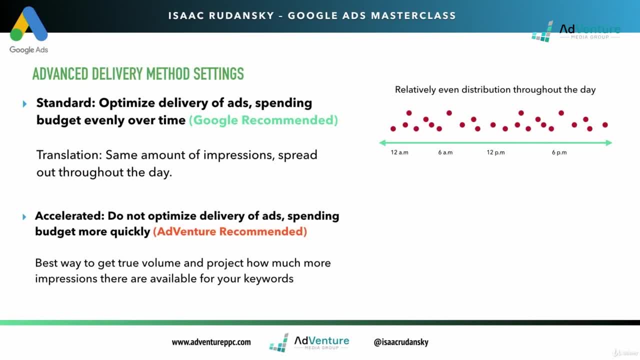 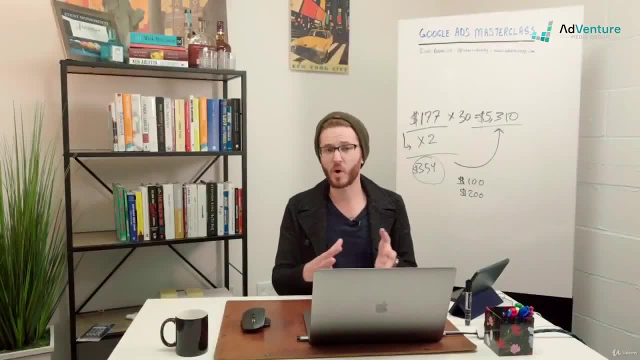 I recommend at Adventure Media. It's the best way to get true volume and project how much more impressions that are available for your keywords. The way I sort of view it, especially in the beginning, is you want to really know what's out there. But if you want to really know how much, 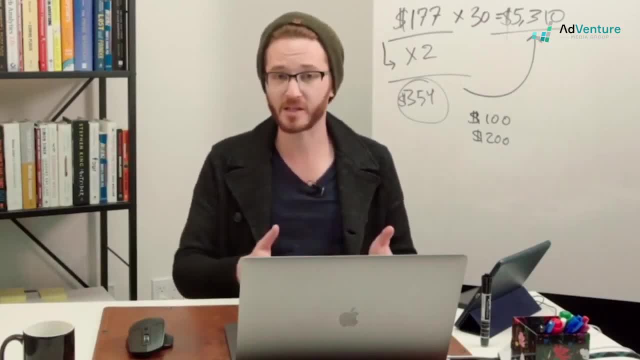 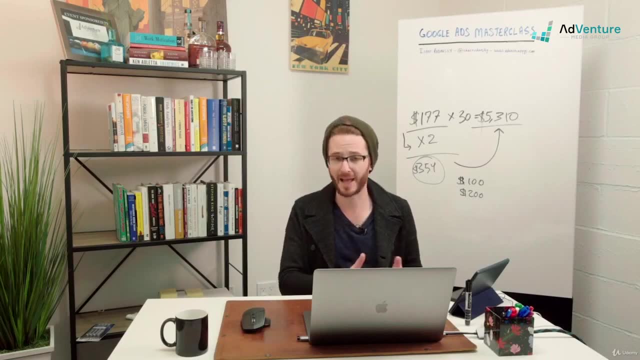 could I spend? you know what? could I really get out of this? Then I recommend accelerated budget. Yes, your budget might be depleted by 10 o'clock in the morning. It might be depleted two hours after your campaign's launched. Fine, And that's not great for. 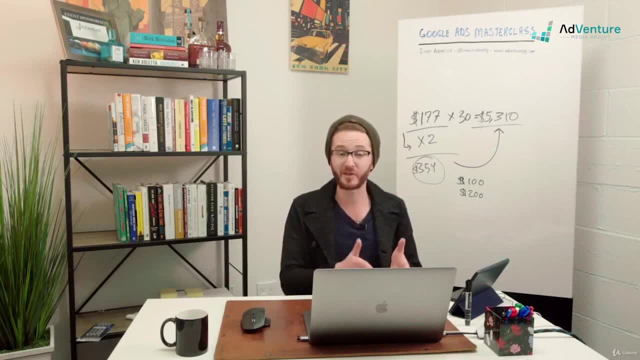 the first day, but it's okay because you're learning. I'm learning that I could spend $50 by 11 am, and what results does that get me? You are missing out on. a really, really important thing is to see do different hours of the day perform differently, which is why you'll have. to eventually adjust: either increase your daily budget, or you could choose to spend $50 or $100, depending on how much you spend, And that's totally fine. You could switch to standard delivery at any point in time in the campaigns. This is an option that could always be changed. 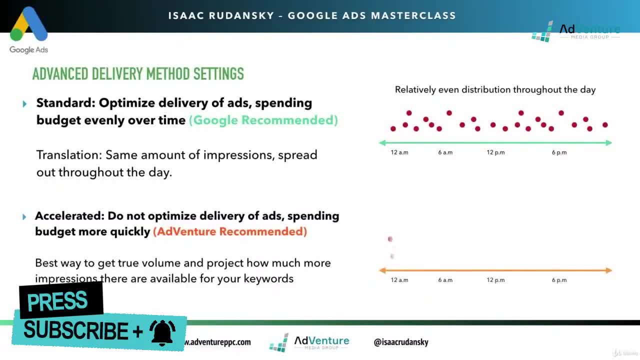 later and just a visual representation of what this looks like If I'm getting all my impressions, and this is what it would look like if I have a lower budget than what I can actually get, based on the maximum amount of search impressions in the locations that 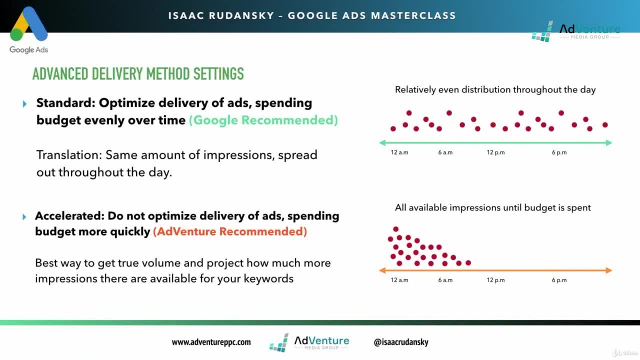 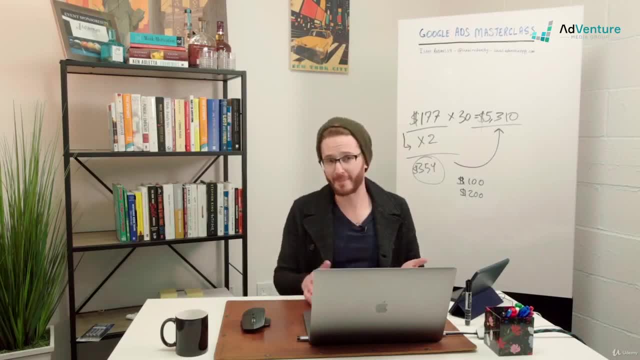 I'm targeting, et cetera, et cetera, And I would have those staggered earlier on. Now, of course, you could choose accelerated and your ads could show all day. And what would be the reason that that might happen is because the combination of two factors, which is my, 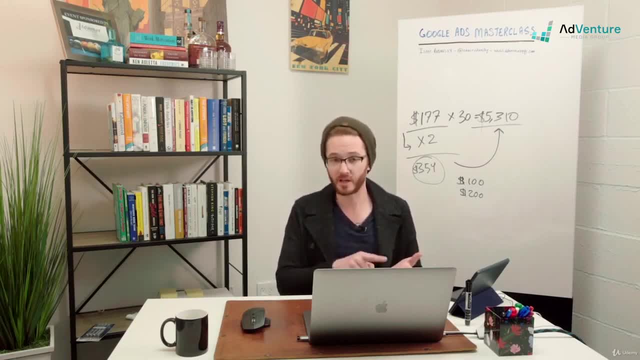 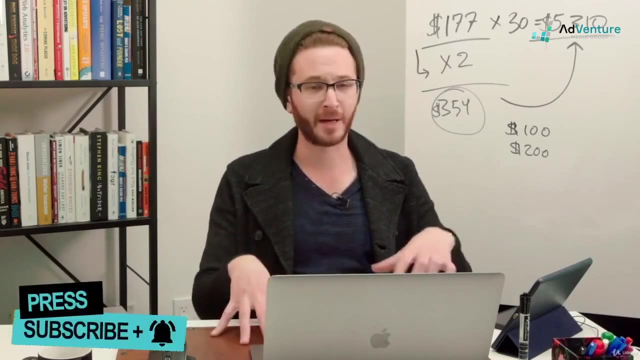 daily budget and the amount of available impressions for a given keyword search term ad group campaign- are enough that my daily budget covers or exceeds the amount of maximum impressions that I can get. And that actually happens more than you'd think, because not every keyword has a huge amount of volume And depending on your match type, depending on your location, 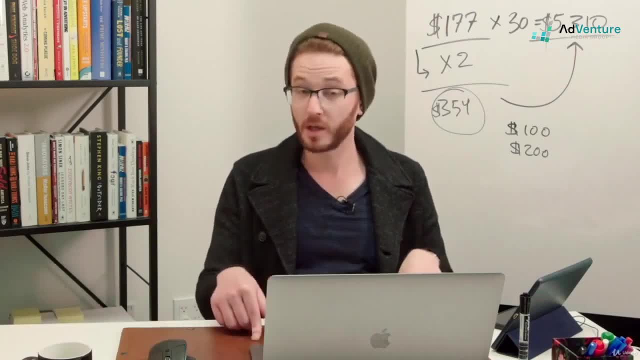 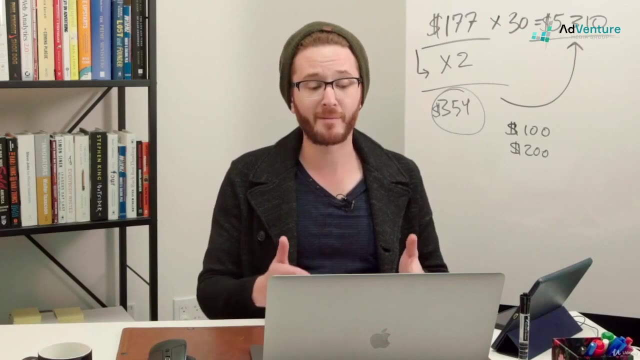 settings but depending on when your ads are scheduled to actually run. So it's quite a common that we'll have a campaign on accelerated budget and our campaigns are running and our impressions are being. we're receiving impressions throughout the entire day, or throughout the entire time we're actually having those ads scheduled to run. So I recommend 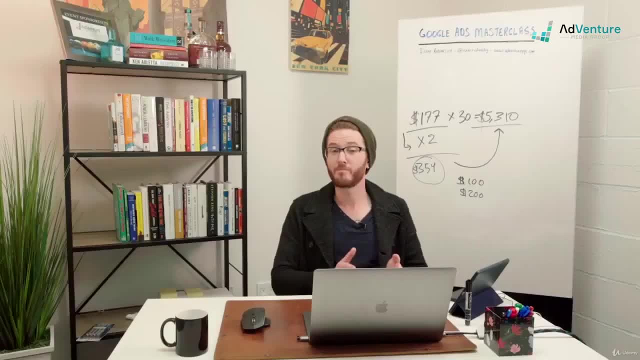 going to accelerated Choosing. accelerated to start Monitor when you start getting less activity and then decide whether or not you want to increase your budget based on profit, of course, based on exposure, based on what your sales team or your website can handle or how the results of the campaigns are going. Of course, that's different for everybody. 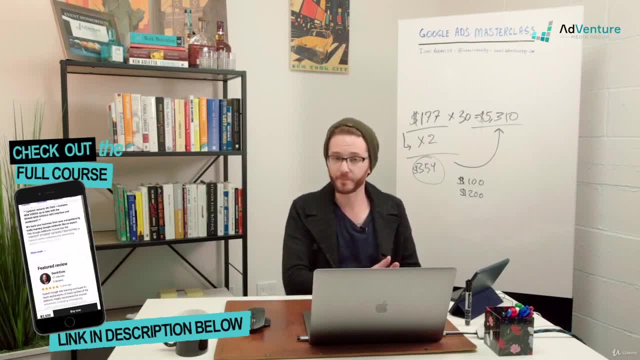 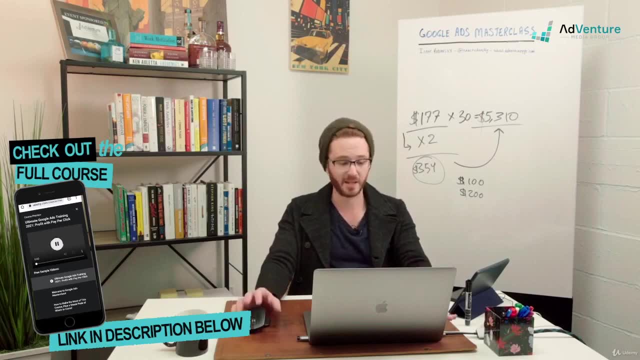 So either change, change, change, Change, choose, choose, choose, choose standard or switch or increase your daily budget. so that's the advanced delivery method settings. let's quickly jump back into into Google Ads and select our settings, the ones that we want to use back in Google Ads. I'm going